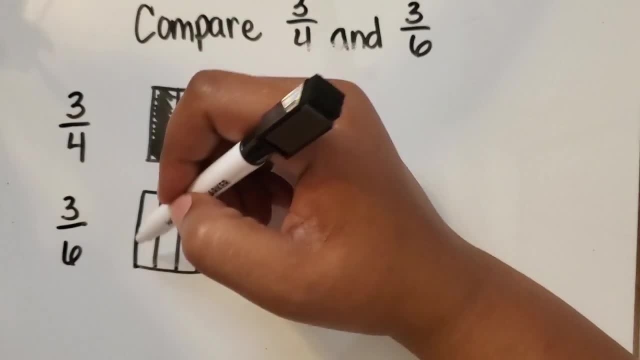 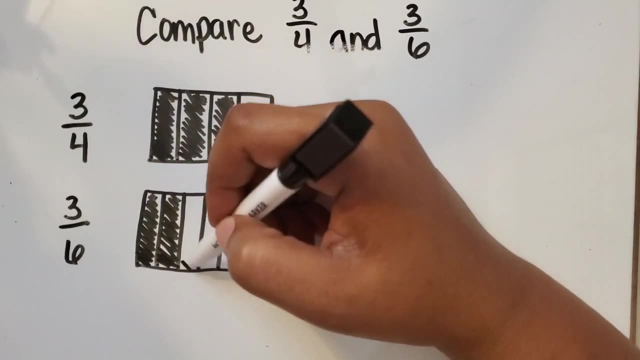 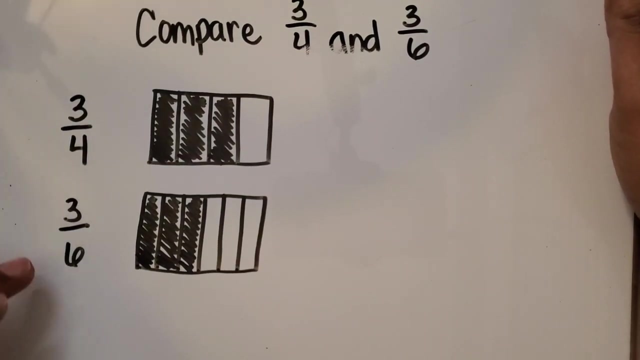 So out of the 6 equal parts, 3 will be shaded in: 1 sixth, 2 sixths, 3 sixths. So let's look at this: 3 fourths compared to 3 sixths- which fraction has a greater value or takes up more space of that whole? 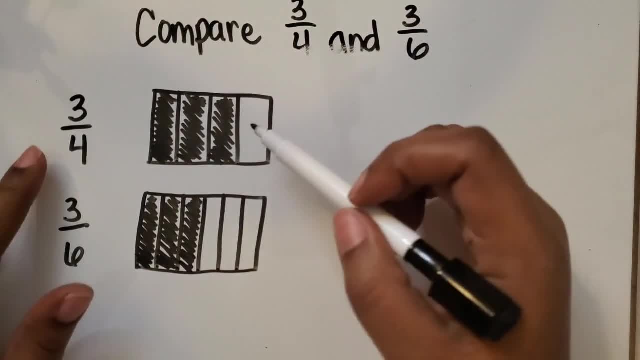 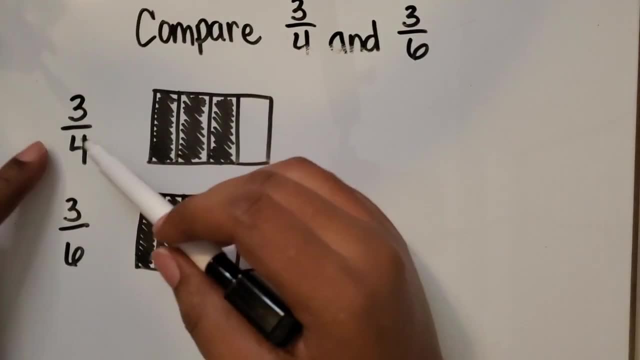 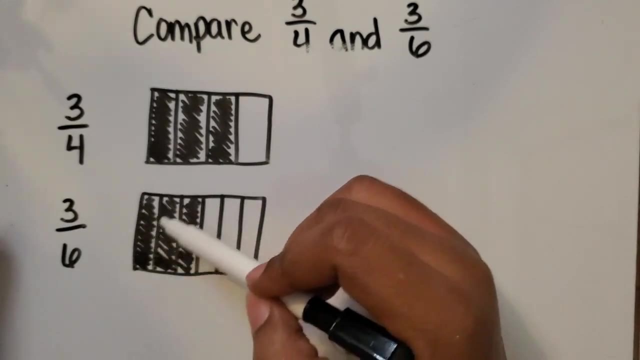 Looking at our models, which are the same size whole, we can see that 3 fourths is a greater fraction or greater value than 3- sixths. Even though the denominator 4, is less than 6,, the size of those fourths is greater than the size of the whole. 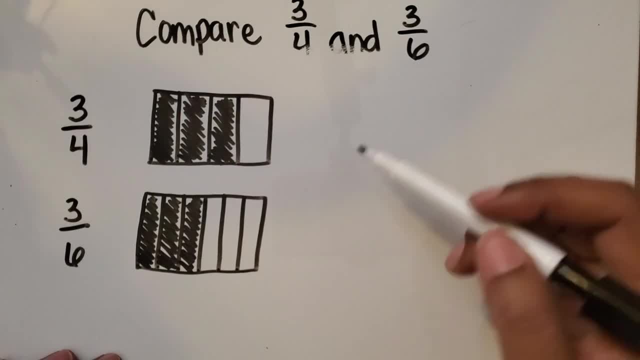 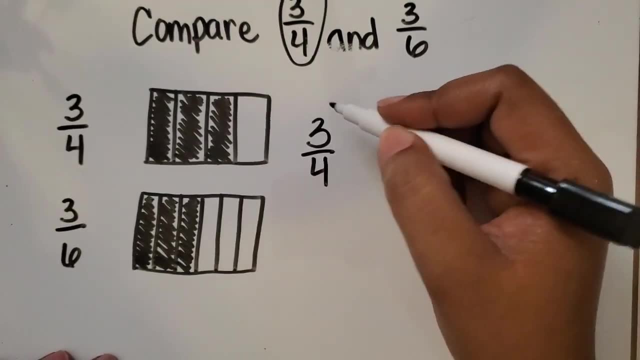 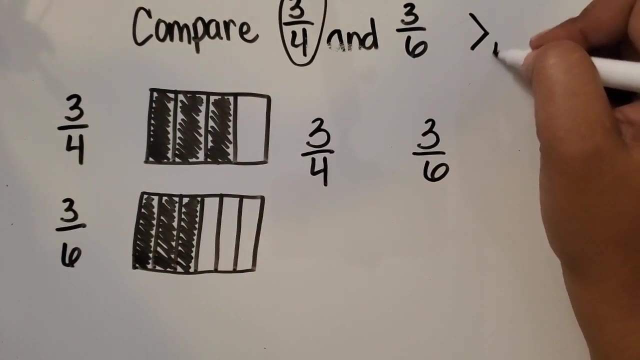 So now we can write our comparison statement. We know that 3 fourths is the greater fraction, So we're going to start with 3 fourths. That was our first fraction, And here goes 3 sixths. So again, which symbol? comparison symbol. 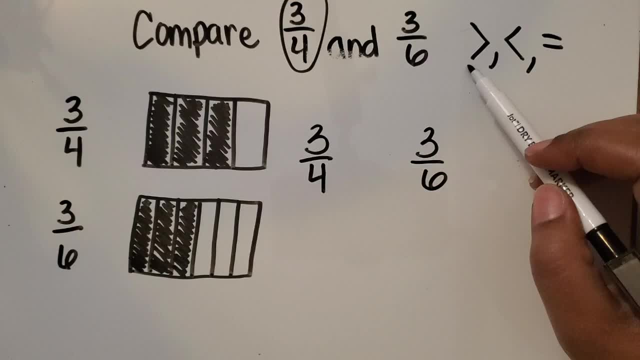 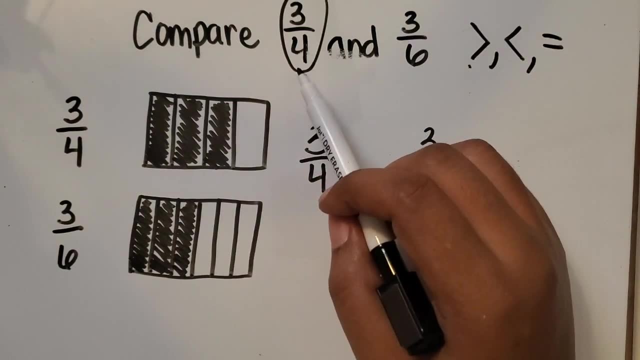 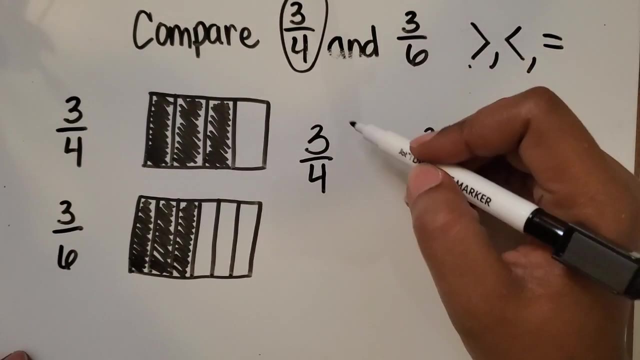 are we going to place between our two fractions, The greater than symbol, less than symbol or equal to symbol. So we know 3 fourths is greater. That's why I circled that one. So I know my symbol is going to face or be open to the greater fraction or the greater value. 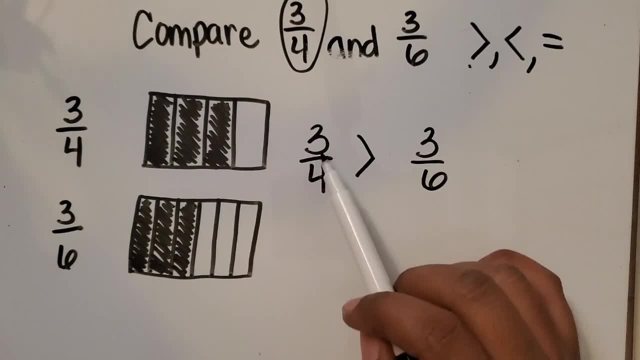 So let's read our comparison statement now: 3 fourths is greater than 3 sixths.